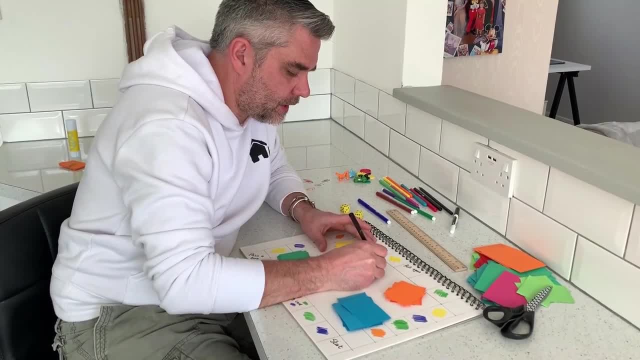 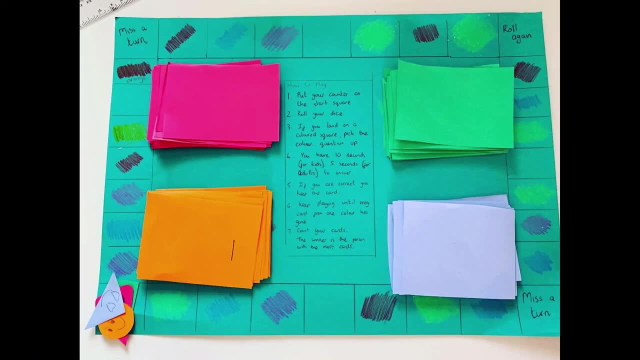 your game so that you know how to play it. So that's what we're going to do next. However, I have already done this with Bella, and these are the rules that we came up together. Writing rules is a really good writing opportunity for children, and there's lots of language. 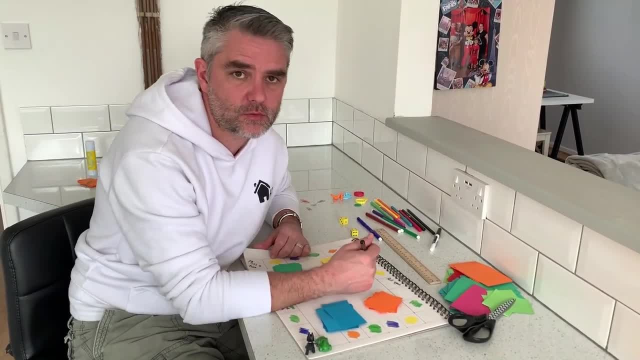 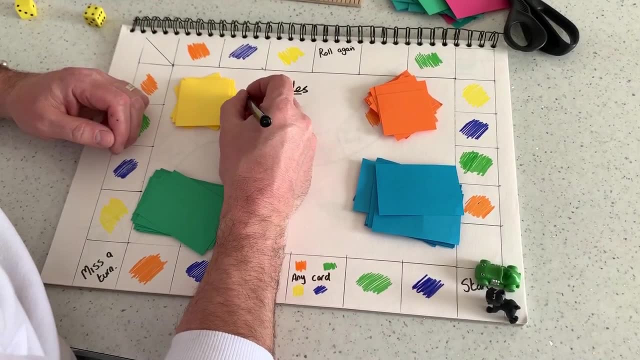 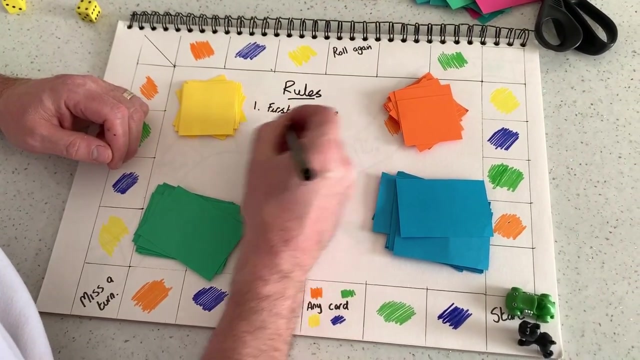 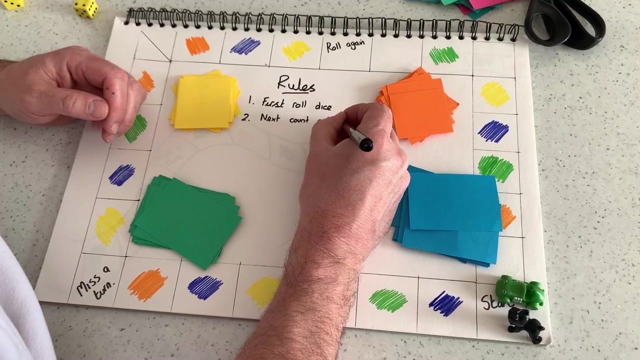 in there you can talk to them about. So I'm just going to have a little go at writing some of the R rules for our game. There's lots of great time words that you can use when you're writing your rules. So for example, first roll the dice, Next count out your. 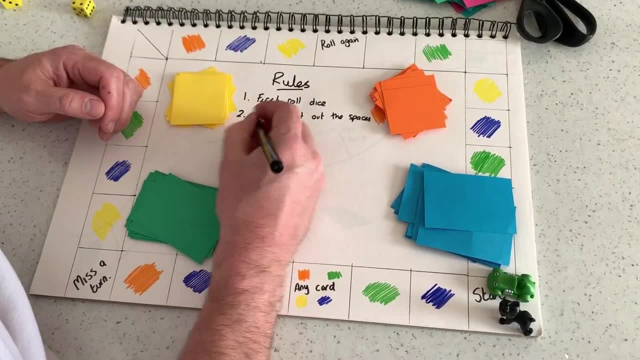 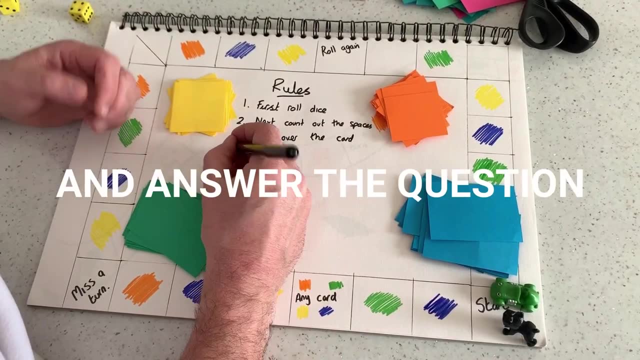 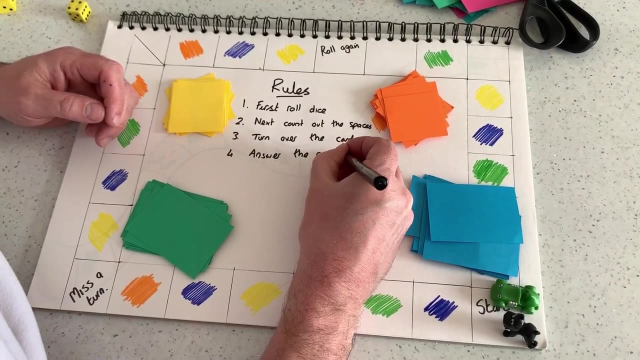 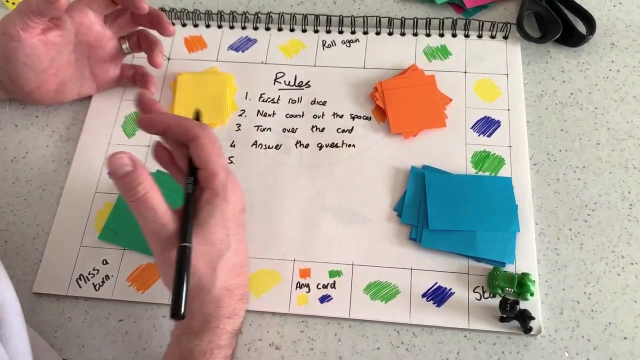 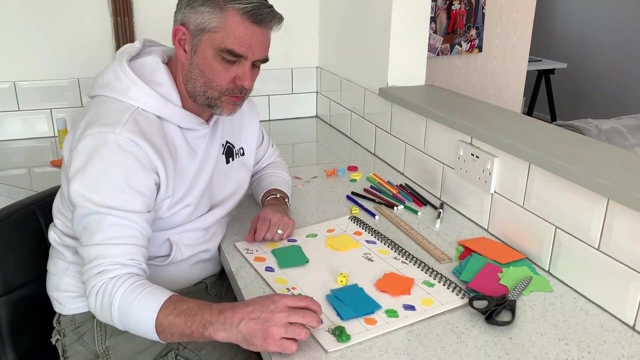 spaces, Turn over the card And answer the question Now. in our game we decided that we would keep the card if we got it right and the winner would be the one with the most cards at the end. Okay, so let's have a go at the game. Take my die roll. it got number two. I'll move. 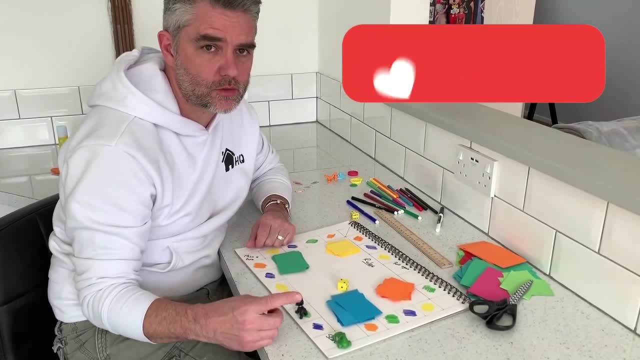 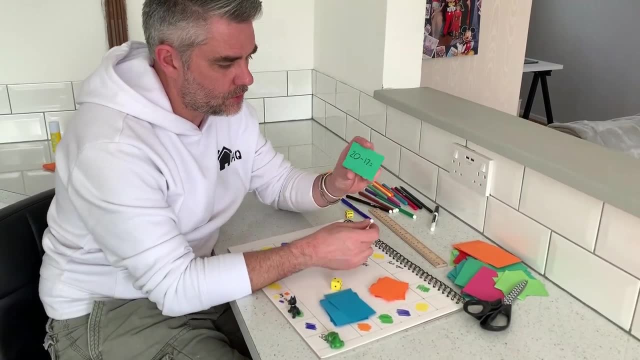 my counting with the dog: One two. always make the children count, always count with them. Daily counting is fantastic. One, two. so I'm on green. I've got my question. Ooh 20, take away or subtract 17.. Now in. 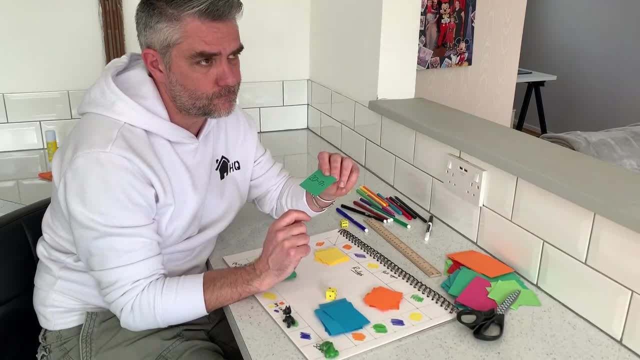 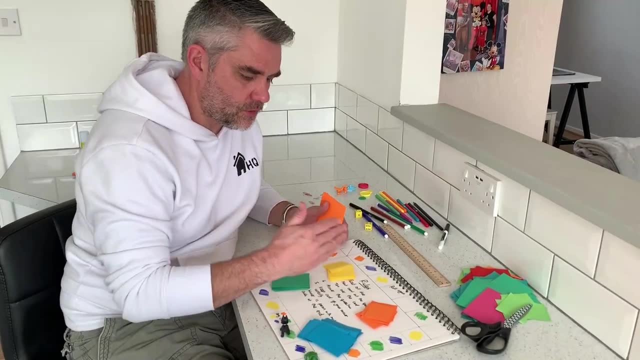 my game. I've got to get that right to be able to keep the card. I know that that answer is three. Check with everyone else. Everyone agrees: I get to keep the card. So this game covers all the four different math operations. but you can adapt these games. 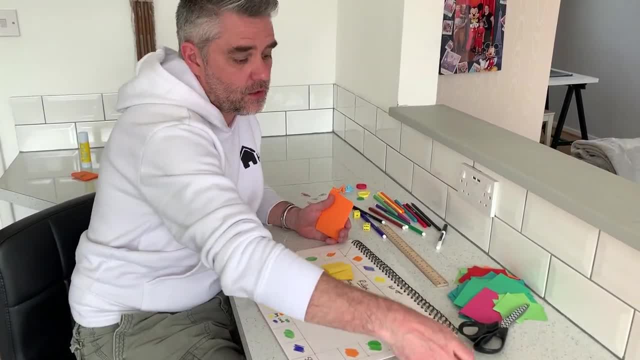 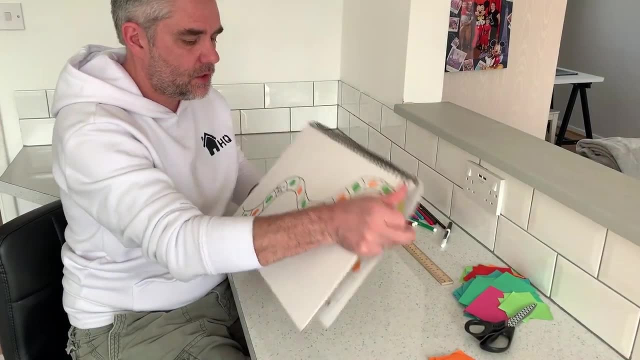 to make them easier for maybe younger children or children who are struggling with certain parts of the maths. For example, you could do one for like number bonds to 10 or to 20.. I've just got a simpler sort of board to play on. I've got 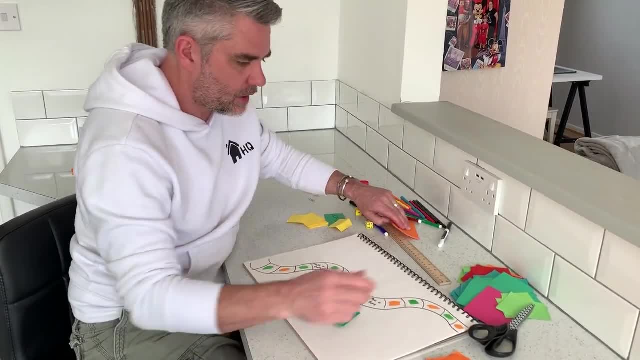 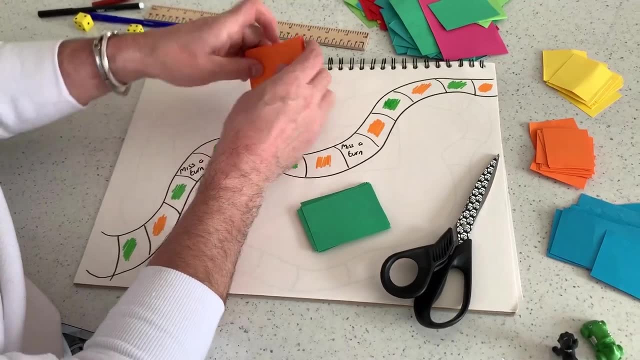 a green one there where I've already done some subtractions and I could make some orange cards with some additions on. So I'm just going to make some cards just to help the children practice with number bonds to 10 or number bonds to 20.. I could just simply.